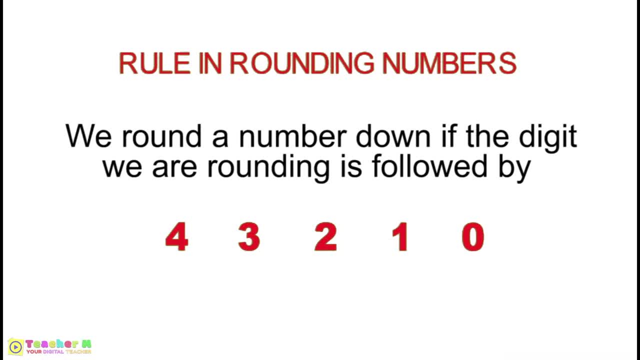 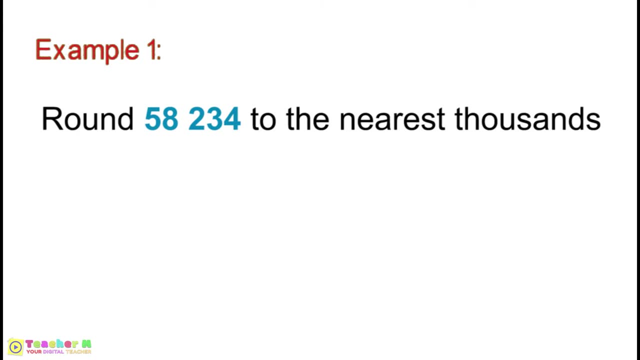 Okay, now what are the steps to follow in rounding of numbers to the nearest thousands? Well, let's take a look at this example, Example 1. Round 58,234 to the nearest thousands. Step 1. Label each digit with the correct place value. 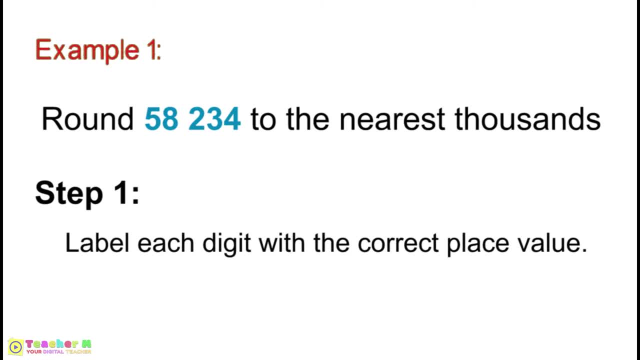 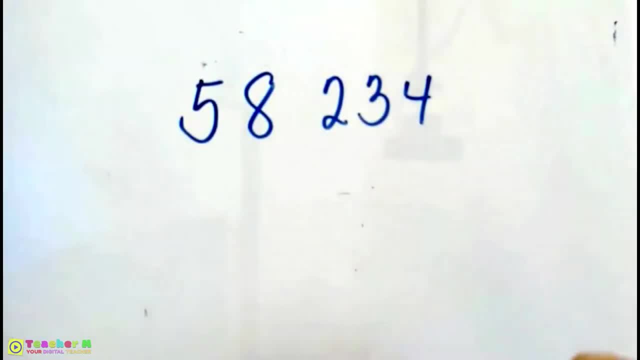 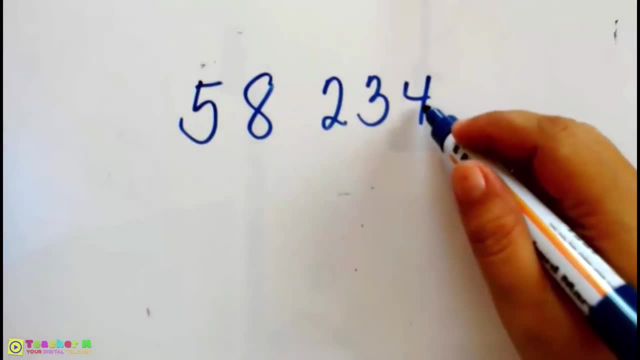 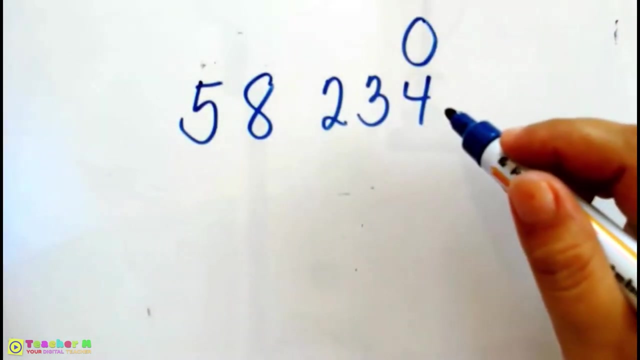 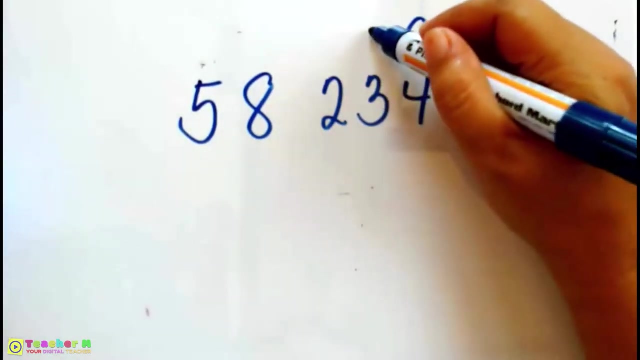 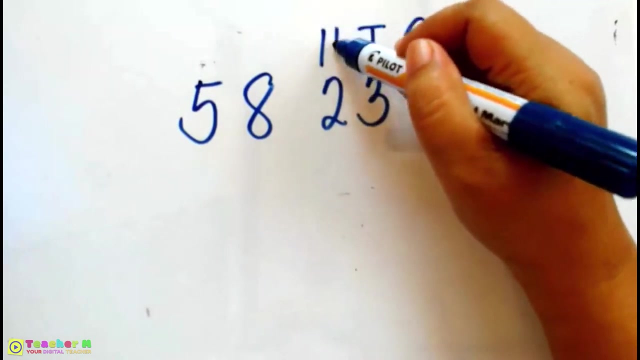 So we will label each digit of the number. We will start from here. 4 is in the once place, I will write letter O for once. 3 is in the tens place, So I will write letter T for tens, And 2 is in the hundreds place, I will write capital letter H for hundreds. 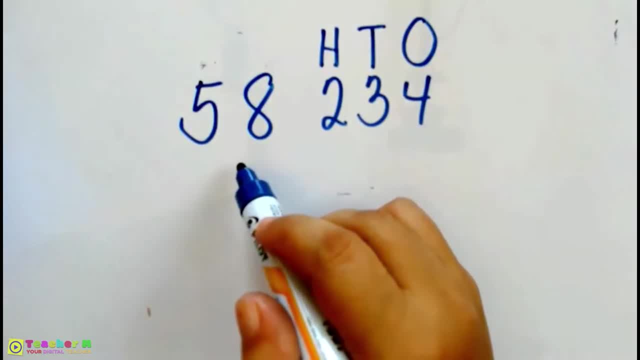 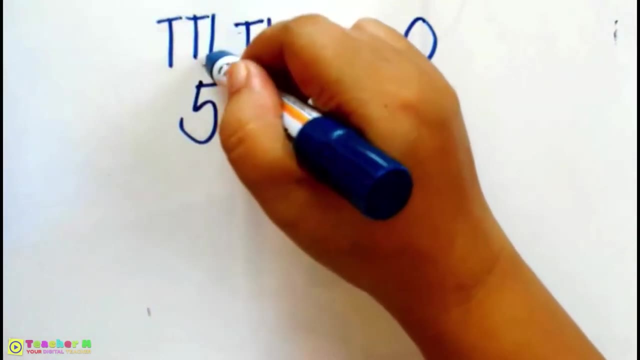 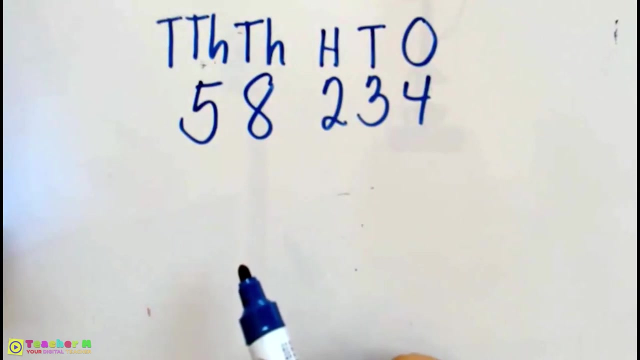 8 is in the thousands place, so i will write th for thousands. and 5 is found in the 10 thousands place, so i will write t t h here, since we're going to round this number to the nearest thousands. so i will underline the place value of thousands. so here, 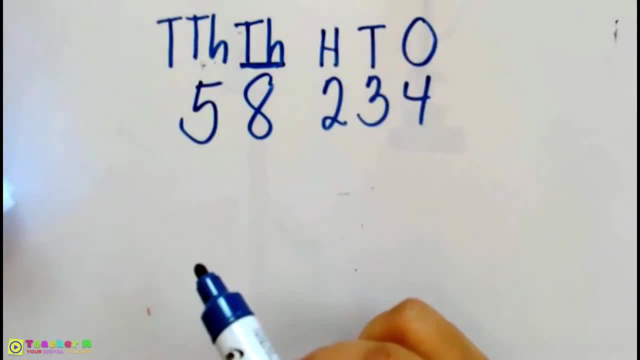 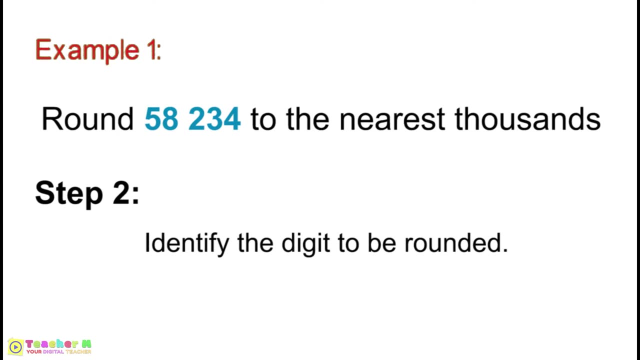 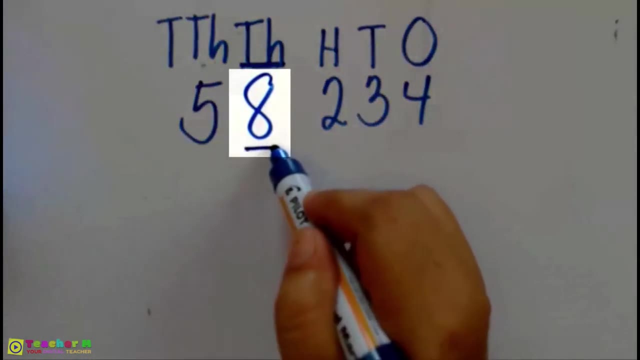 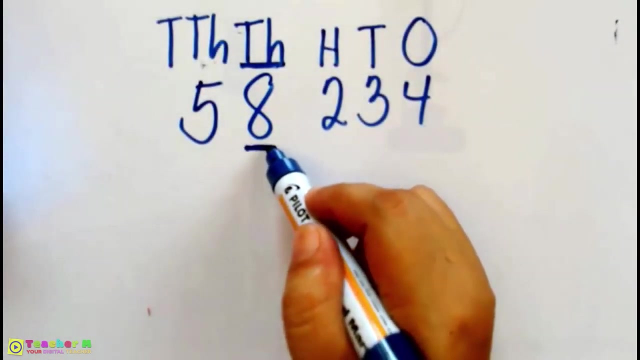 after labeling each digit with the correct place value, we will now do step two, which is to identify the digit to be rounded off. and the digit to be rounded off here is eight. why eight? because we are going to run this number in the thousands play. so eight is the digit found in the thousands place. 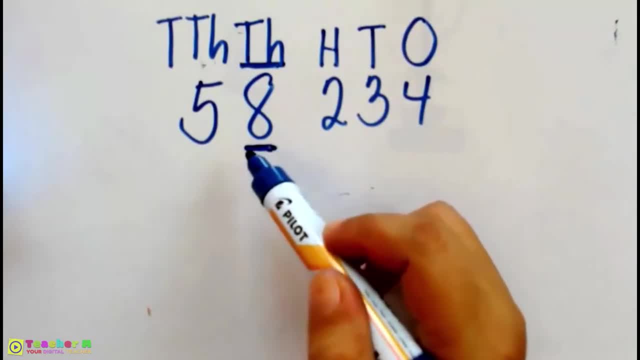 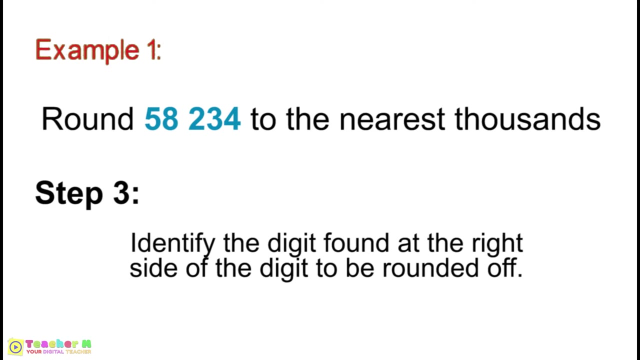 so, as you can see here i underlined eight, so we will have a guide that this is the digit that we will round off. okay, after identifying the digit to be rounded off, let's do step three, which is to identify the digit found at the right side of the digit to be rounded off. 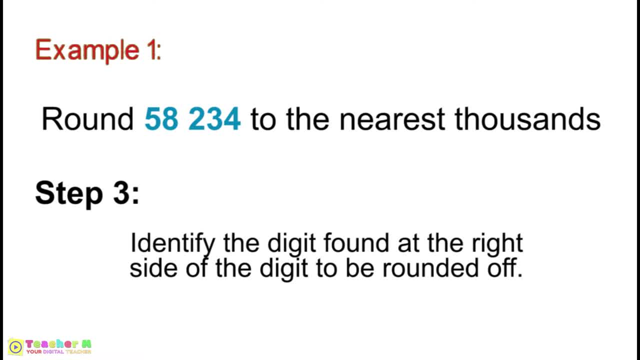 and always remember that if the digit to be rounded off is followed by five, six, seven, eight or nine round up, and if the digit to be rounded off is followed by four, three, two, one or zero round down, what digit is found at the right side of eight here? 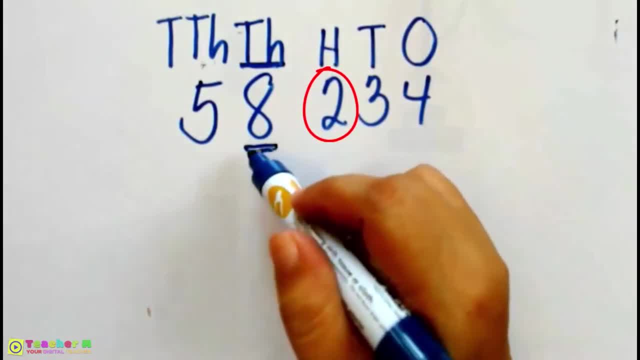 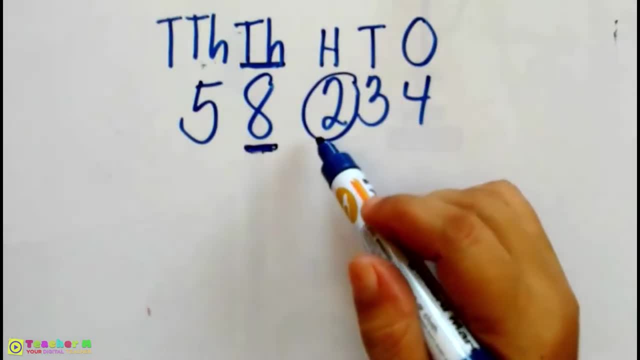 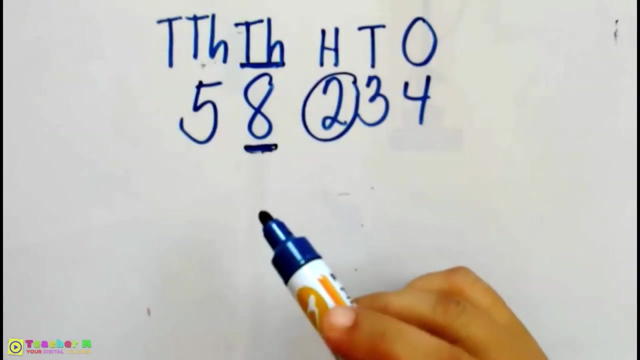 you are correct. the digit found at the right side of eight is two. so eight here is followed by two. we are rounding here is followed by two. so we will round down. when we round down, we just copy the digit we are rounding. so we will copy eight here. okay, let's copy eight, since eight is. 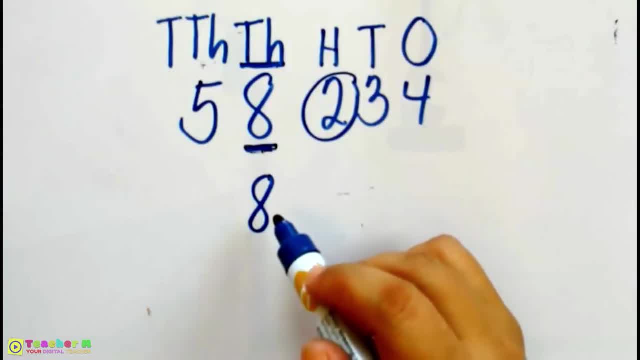 the number we are rounding and then what's the next step that we're going to do? we will do step four, step three, which is to change all the digits to be rounded off, to be rounded right to being round up to the middle part. number four include sign, ok will interview from the number six towards the productivity of sevencre, pertinent of nine to be rounded down. and you will need to find the absolute digit of a hand styleace from the hand style tears options to the right hand side to be rounded off: birth chart, and you will slip sauce. otherwise you need two practice on certain date in business process you can get open on the top right. so to repeat these numbers, you have to complete all the digits and AudioCAD. 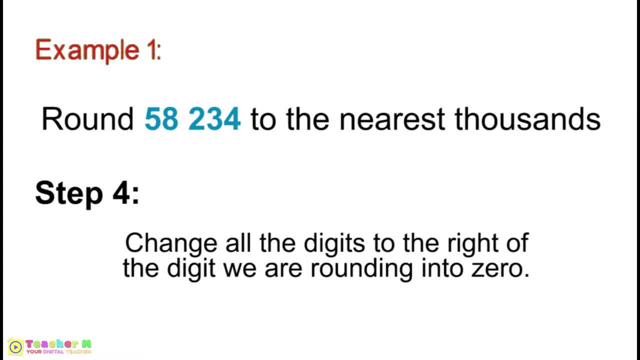 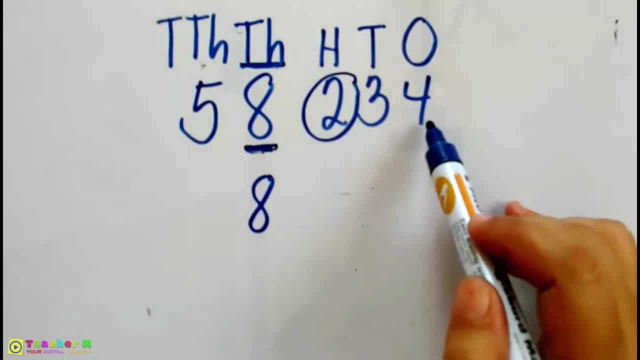 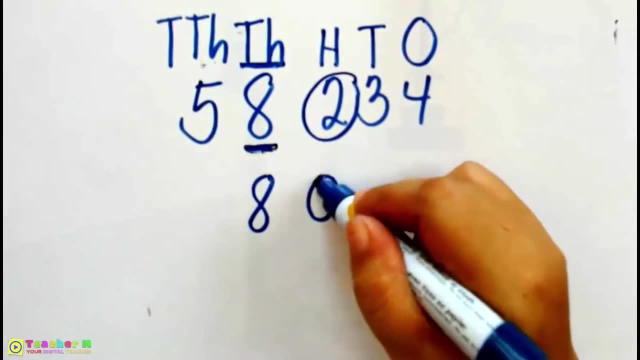 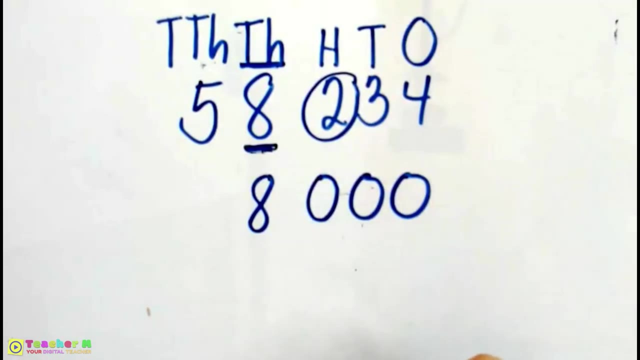 digits to the right of the digit we are rounding into zero. so since there are three digits here, which are two, three and four, we will change all these digits into zero: two will become zero, three will become zero and four will become zero. then we will do the last step, step five, which is: 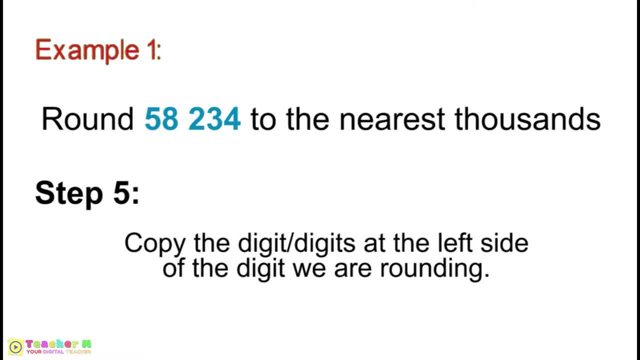 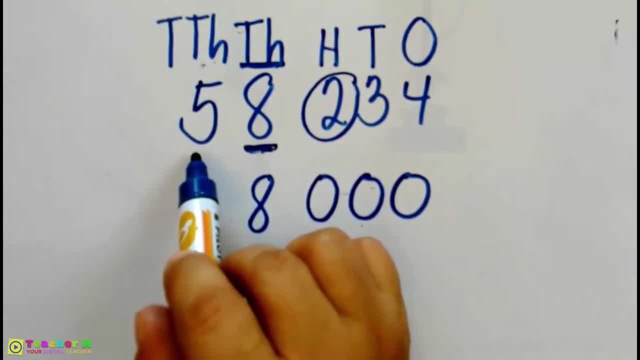 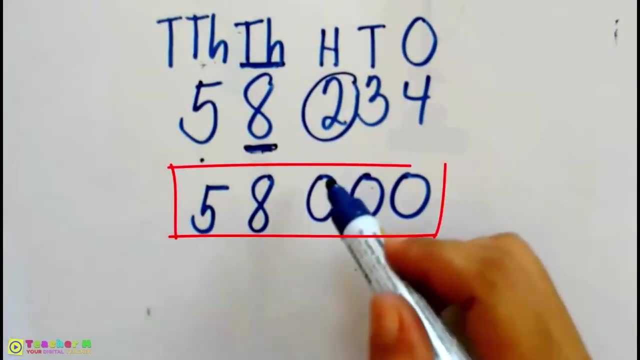 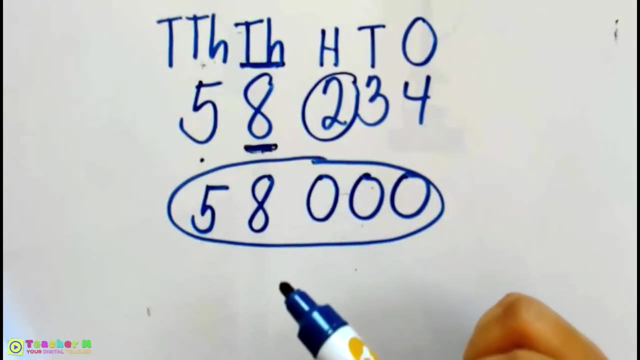 to copy the digit or the digits at the left side of the digit we are rounding, since there is only one digit at the left side of eight, which is five, so we will write five here. so our answer here is 58 000. so if 58, 234 is rounded off to the nearest thousands, the answer is: 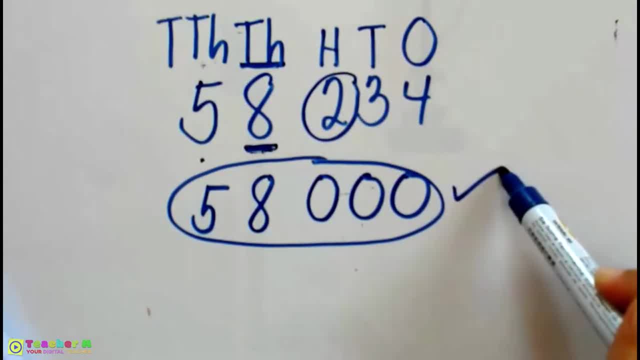 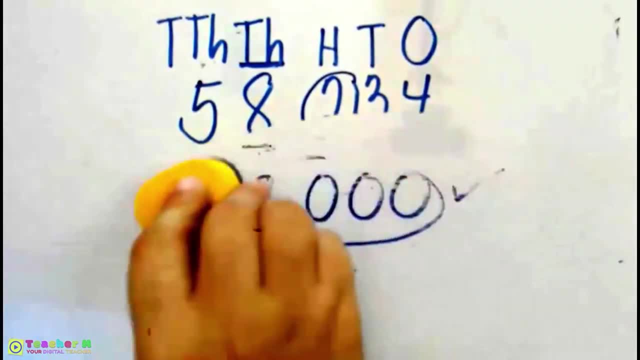 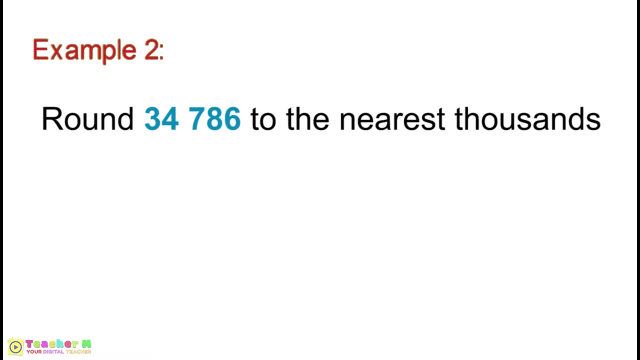 58 000. okay, now let's take a look at our next example, example two. okay, let me erase this one. first example two, round 34 786 to the nearest thousands. step one: label each digit with the correct place value. so we will label each digit of the number 34 000. 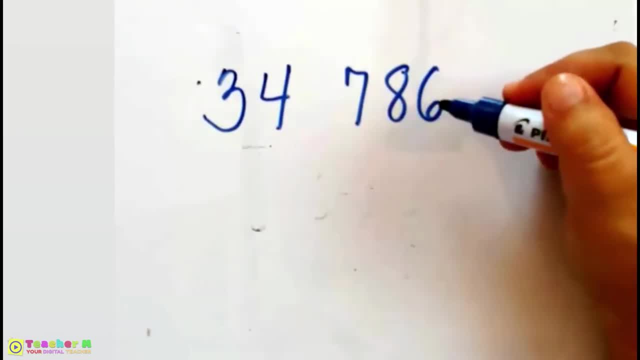 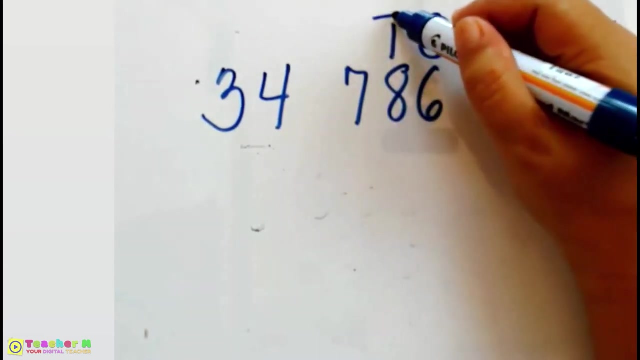 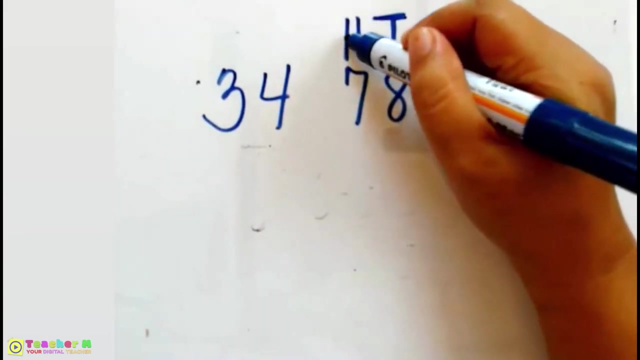 786 with the correct place value, so we will start from here. six is in the ones place, so i will write o for once. eight is in the tens place, so i will write t for tens. seven is in the hundreds place, so i will write h for hundreds. four is in the thousands place, so i will write the h for. 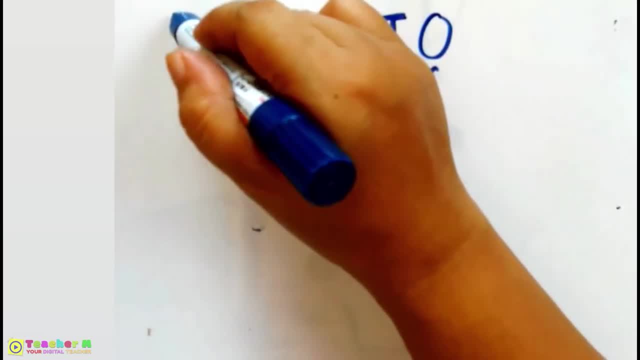 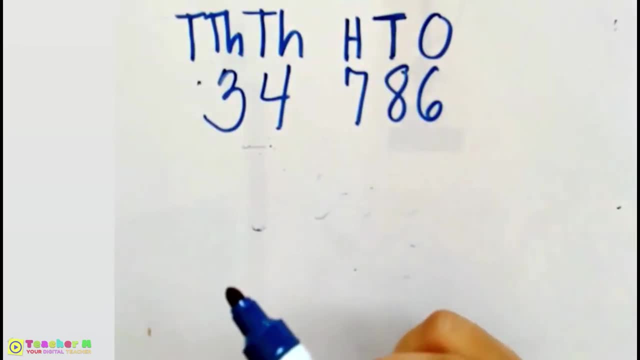 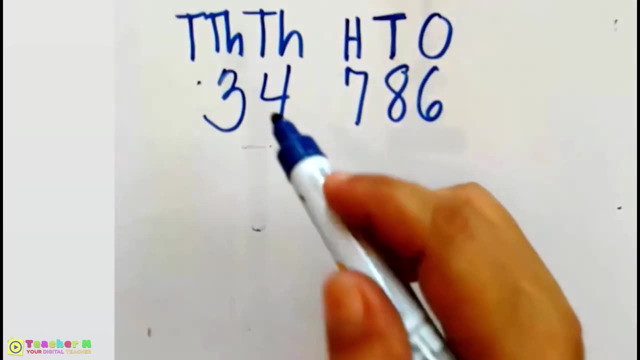 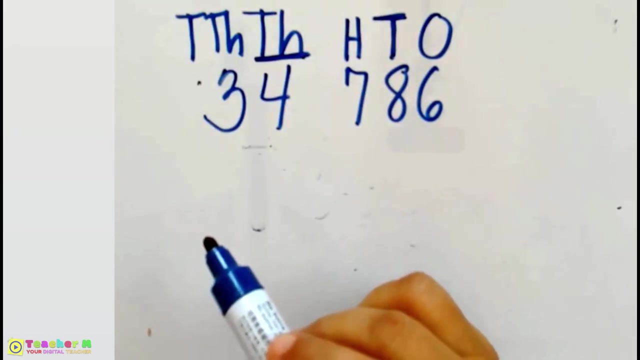 thousands and three is in the ten thousands place, so i will write tth for ten thousands, since we're going to run this number to the nearest thousands, so i will underline the place value of thousands here. okay, thousands. after labeling each digit with the correct place value. 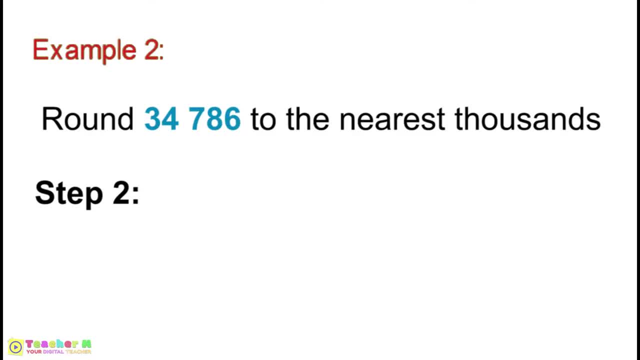 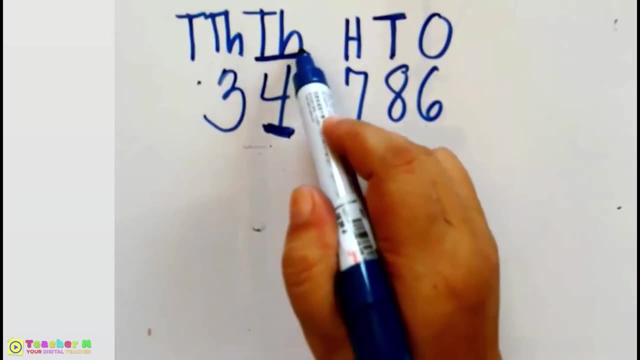 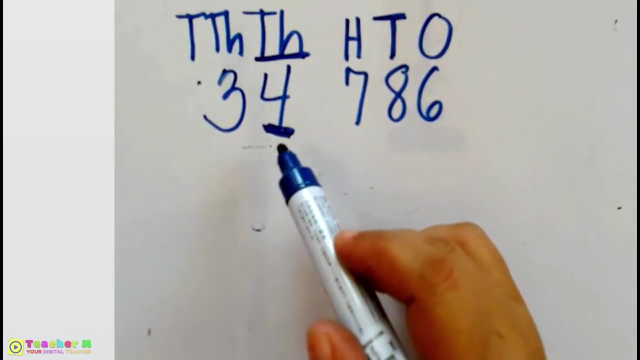 we will now do step two, which is to identify the digit to be rounded off. the digit to be rounded off here is four, because four is in the digit found in the thousands place. okay, so we will underline four, so we will have a guide that this is the digit to be rounded off. okay, since we have already 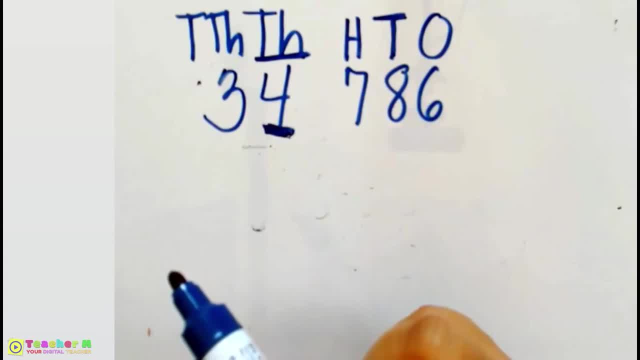 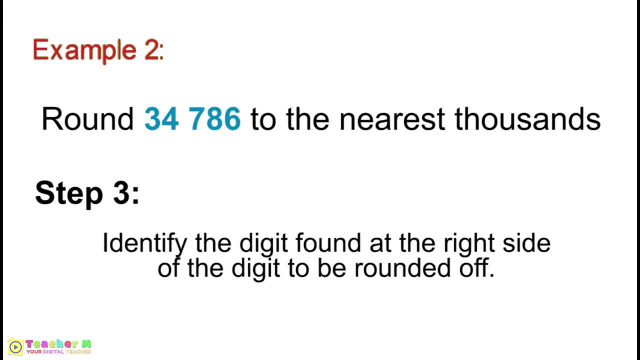 identified the digit to be rounded off. we will now do step two, which is to identify the digit to be rounded off. let us proceed with the next step, step three, which is to identify the digit found at the right side of the digit to be rounded off. and always remember that if the digit to be rounded off is followed by 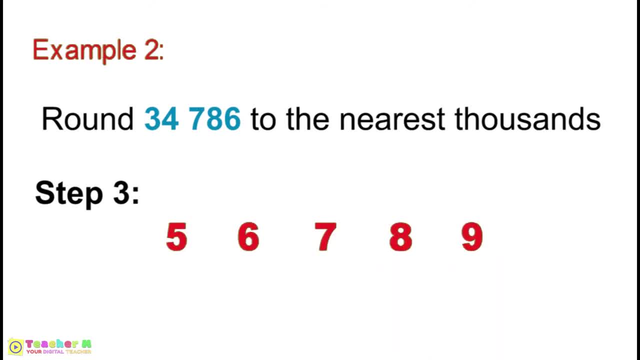 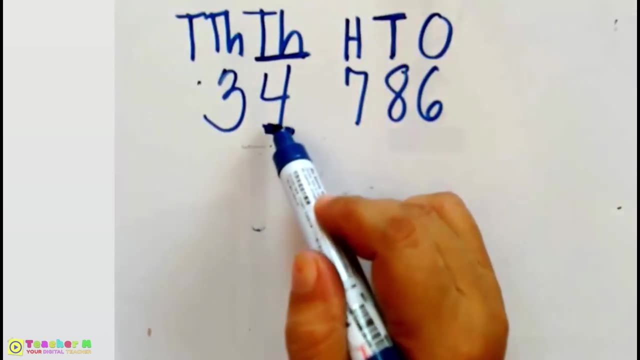 five, six, seven, eight or nine, round up correct. and if the digit to be rounded off is followed by four, three, two, one or zero, round up down. Since 4, here the digit we are rounding is followed by 7.. Okay, so 7 is found at the right. 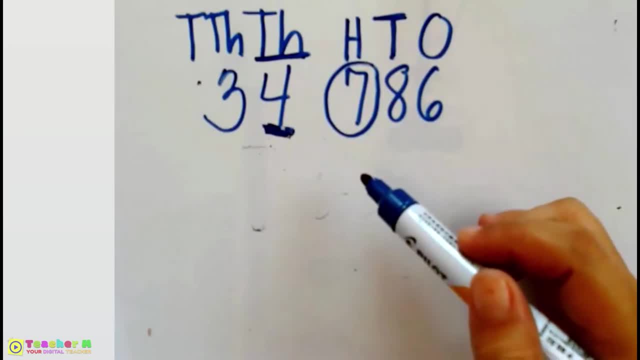 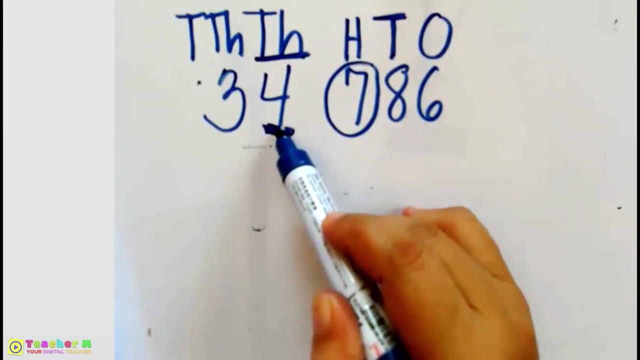 side of 4.. So we will round up, Correct. So what are we going to do now, Since we're going to round this number up? Okay, we will add 1 to the digit we are rounding, which is 4.. So we will add 1 to. 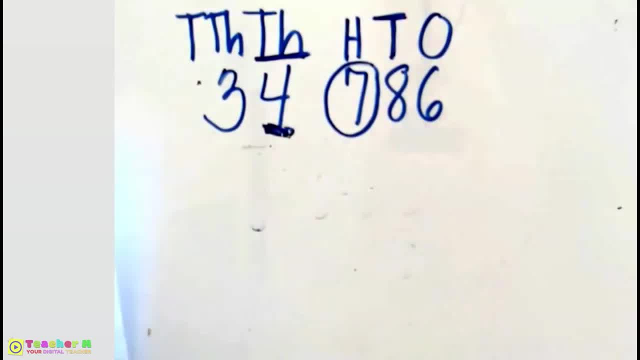 4.. So I will rewrite this number here. This one, 34,786.. And 4 is the digit that we're going to round off. Okay, so we will now round this number up, Because the number that follows 4 or the 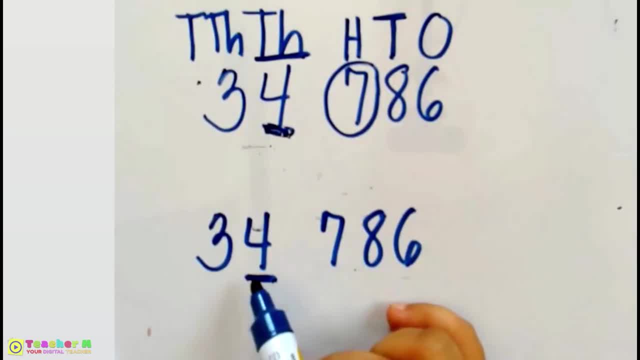 number found at the right side of 4 is 7.. Okay, so 4 plus 1.. 4 plus 1 is equal to 4 plus 1. 5. Okay, And then the next step that we're going to do is to change all the digits to the right of. 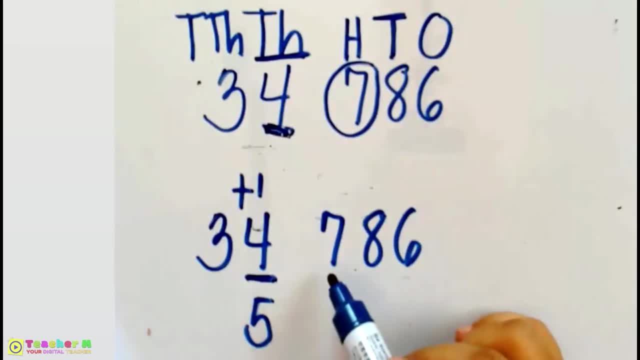 the digit we're rounding into 0. Since there are 3 digits here, which are 7,, 8, and 6.. So we will change all these digits into 0.. 7 will become 0,, 8 will become 0, and 6 will become 0. And then 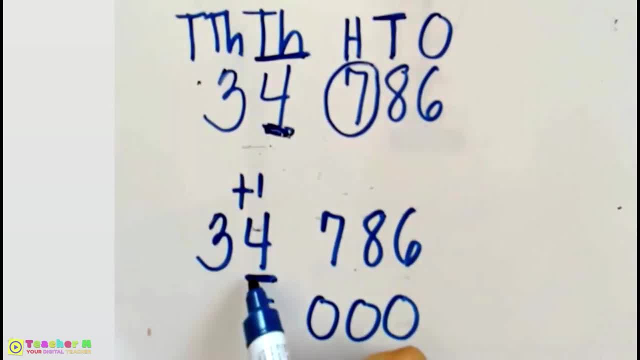 we're going to copy the digit at the left side of 4 here. So we will copy 3 here, because there is only 1 digit here, which is 3.. Okay, so our final answer here is 35,000.. So, if we're going to round, 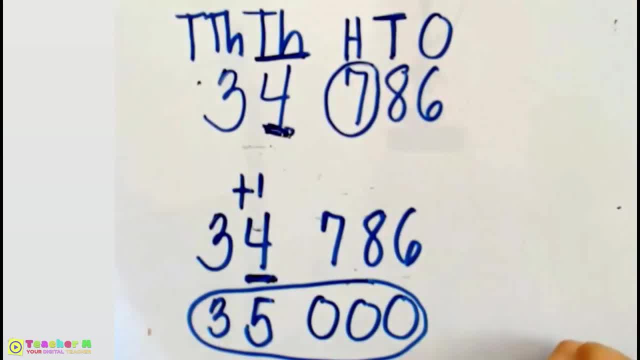 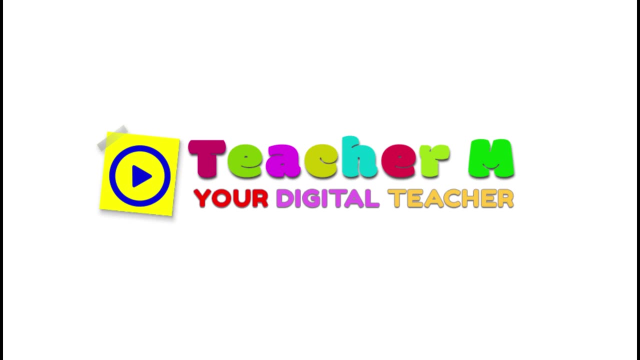 off 34,786. into the nearest thousands, the answer is 35,000.. Okay, so that's all for today. Thanks for watching. This has been your teacher Em saying: keep learning, keep growing. Bye.